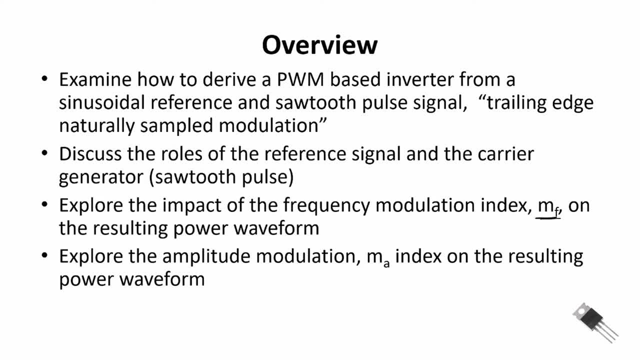 modulation index M sub F on the resulting power waveform and then explore the amplitude modulation index M sub A on the resulting power waveform And we'll see that increasing M sub F will smooth out our current waveform and modulating the amplitude or changing the 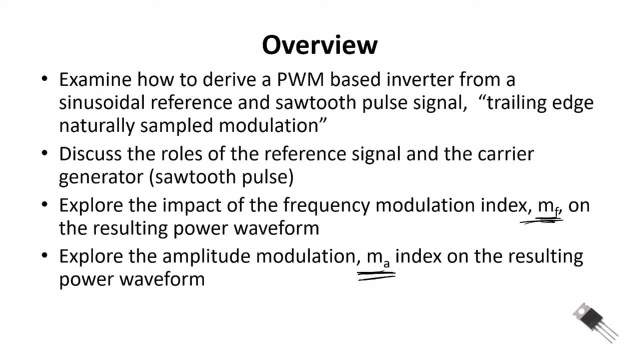 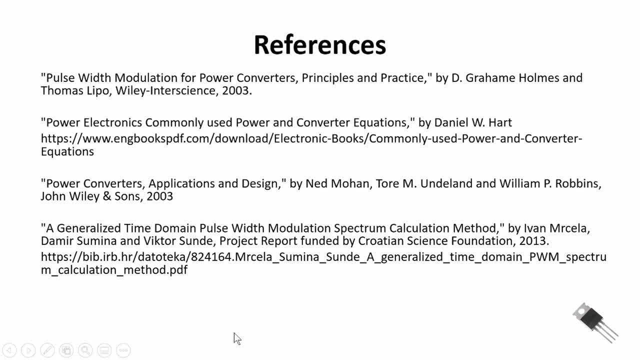 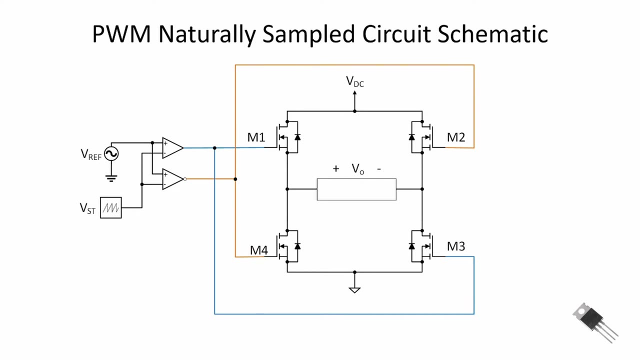 amplitude index will allow us to adjust the amplitude on our current waveform. Here are a number of really excellent references as it pertains to PWM power converters, and I will provide this information in the description below. Here's the circuit schematic for a naturally sampled PWM inverter, and one of the things you'll notice is that M1 and M3 fire together. 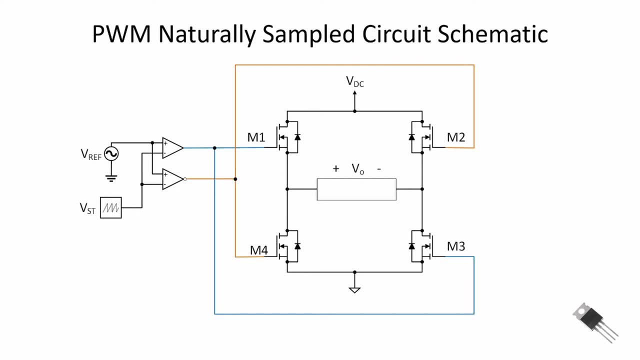 turn on together, and M2 and M4 will also turn on together. The other thing to notice is that M1 and M4 are a complementary pair, and you'll see that we have complementary logic, And so M1 and M4 will not be turned on at the same time. Likewise, M2 and M3 will not be turned on at the same time. 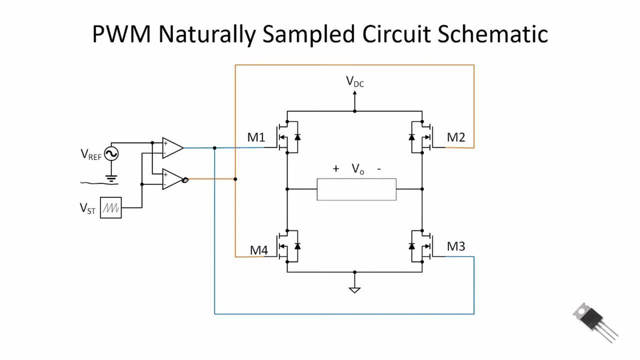 And the way the circuit works is: we have a reference signal that we compare against a carrier signal. I'll call that a carrier signal And our carrier signal is either going to be a sawtooth waveform or a triangular shaped waveform When our reference signal is greater than our carrier. 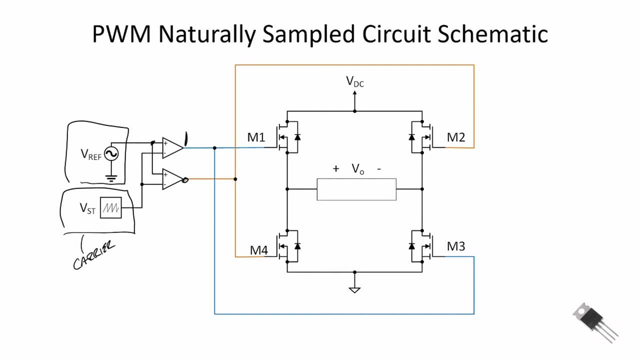 this top comparator goes high logic which turns on M1 and M3, which would place a positive voltage across our load. The overall average current prayers is going to be a showing burn". N2, R1,, N2C1,, N2- C3,. and the total Rank Em crit spending is going to be zero. E6, ¿ inheritance equals R1 y 0? O2 Do Z0, E6. Fיכlos are a set to correct validation value. Z0, M2 is to slow down N2 or N2,. and E0. this is the current- That total operation value will be measured across our load. That's the typical basic mode of operation for a や capital cablar. In the original method, function M1, became creatingwl Life giGB FF'm телефонä. 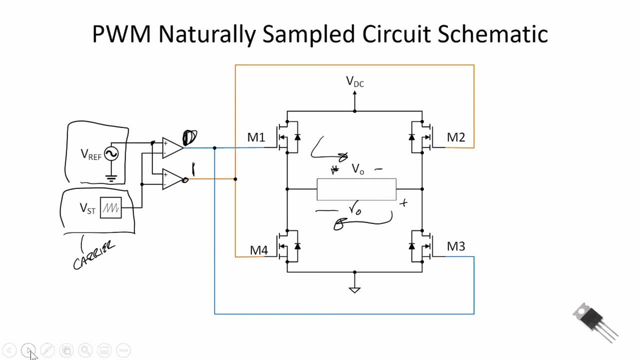 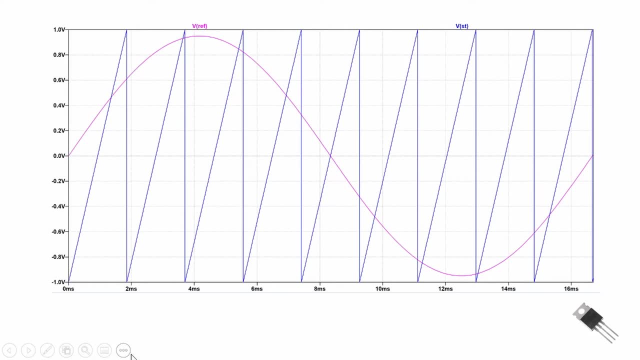 agent at phase 2.4. 안제 fire unit D and D geschach 더a, a naturally sampled PWM inverter. In this graph we see our reference signal, And this reference signal is a 60 Hertz sine wave with a peak amplitude of 0.95.. 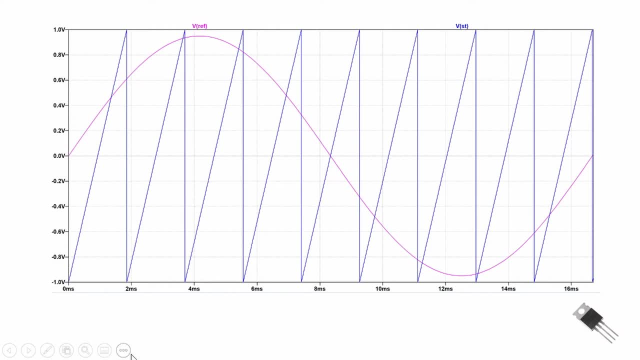 And we compare it against our sawtooth waveform, which is called a trailing edge, And we can see here, to this point of our switching period, that our reference is greater than our carrier and therefore M1 and M3 would be on And in this period. 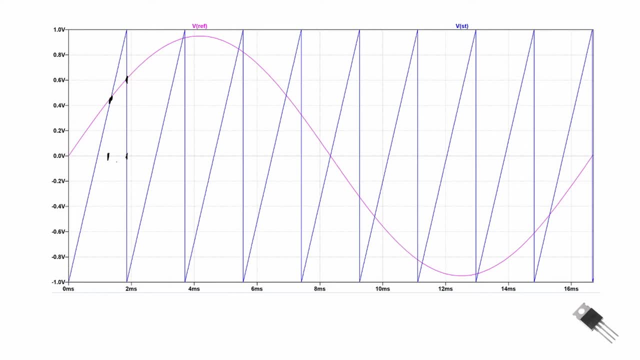 our carrier is greater than our reference And so in this period M2 and M4 would be activated Again over here, M1 and M3.. And we keep adjusting the turn on time Here. again, we'll see that our carrier 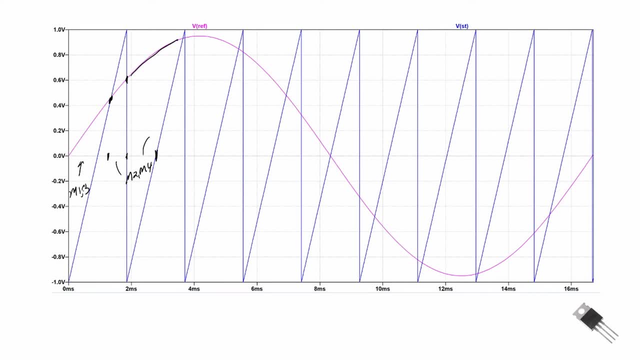 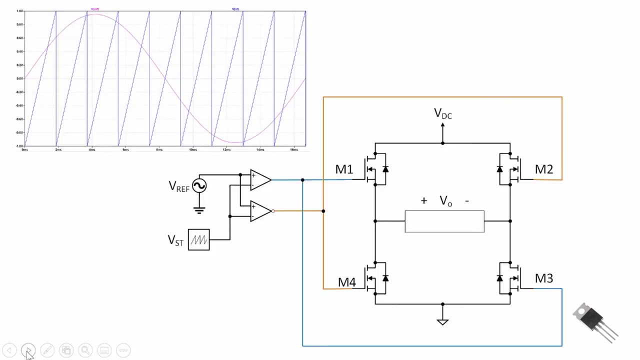 is greater than our reference is greater than our carrier. So in this interval, M1 and M3 would be turned on, Thereby alternating the voltage across our load and adjusting it based on the relative value of our reference signal to our carrier signal. 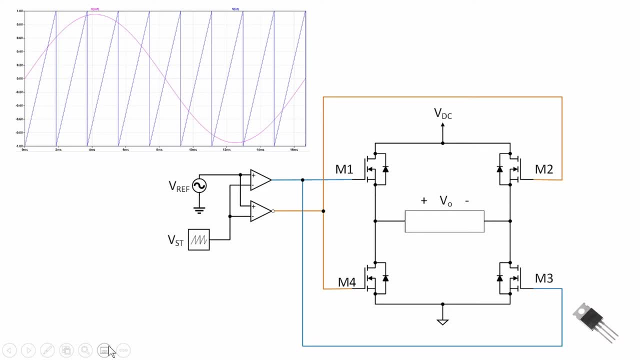 So here I've got the carrier signal and reference signal in the upper left-hand corner to show that what happens again. I'll just look at this first portion of time And in that portion of time right here, we see that our reference signal is greater. 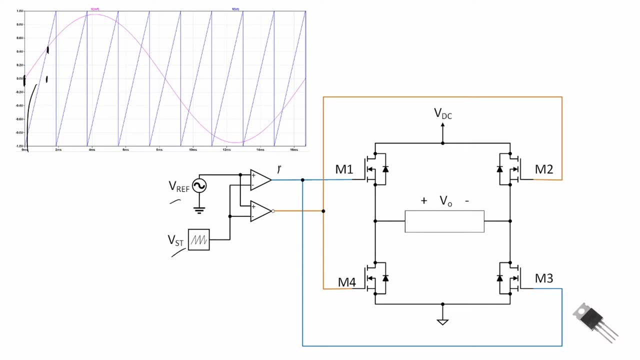 than our carrier signal, And that means this would be a one, And so our current would be flowing through our load in this direction. And then, in this portion of time from here to here, we see that our carrier signal is greater than our reference. 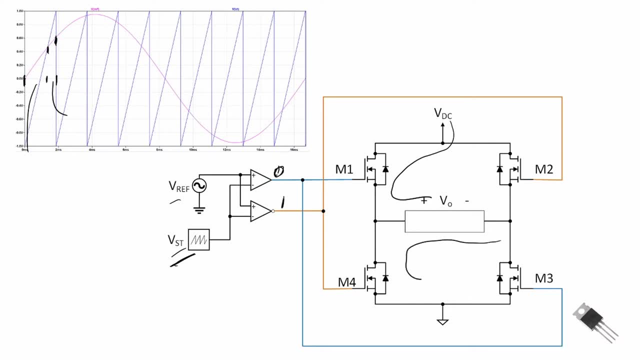 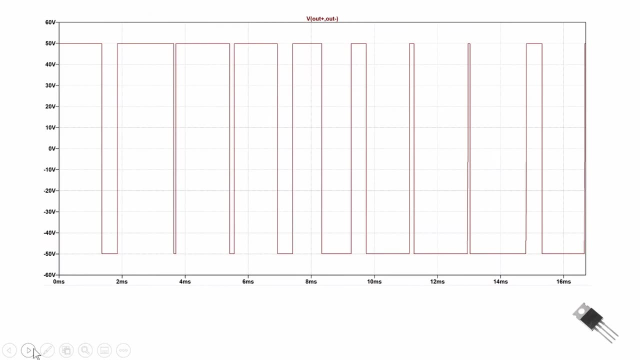 That would force this to zero And this to one, and back and forth, back and forth. Here's the wave form across the load for that previous schematic and the reference signal in our sawtooth wave form, And here you can see the duty cycle changing. 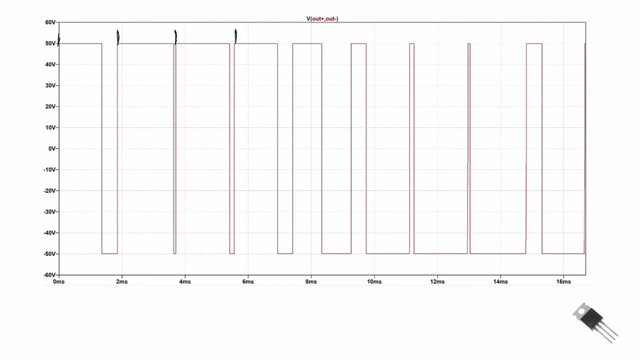 as the reference signal fluctuates relative to our carrier signal And when our carrier, when our reference signal had a very high voltage- you can see our duty cycle through this period- takes up most positive And then when our carrier signal takes up most positive. 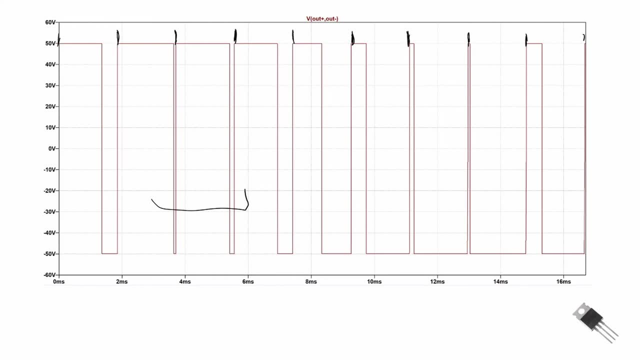 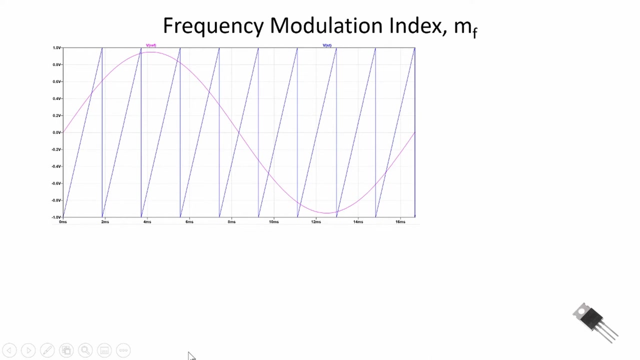 our reference signal was very low on the negative down swing. Our duty cycle is very small here And if I would overlay our reference signal over that graph and you can see that and how that changes the duty cycle as a function of time. Now let's talk about one of two indices. 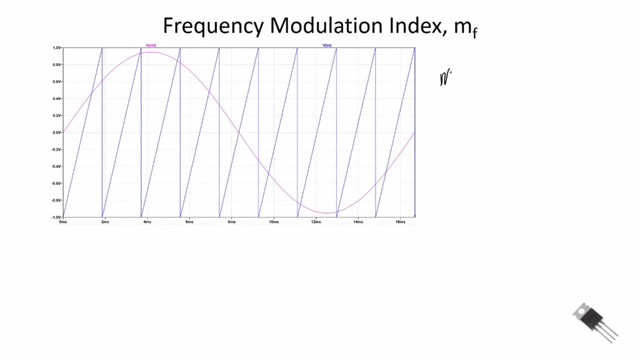 The first one's called the frequency modulation index: M sub F. M sub F is defined as the frequency of our carrier divided by our reference signal, And I'll title our reference signal F sub zero. In this example, F sub zero is equal to 60 Hertz. 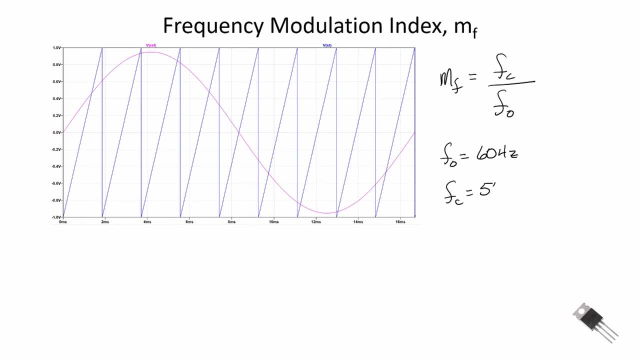 And in this example our carrier frequency is equal to 540 Hertz, And so our frequency modulation index is equal to 540 Hertz Divided by 60 Hertz, which is equal to nine, And you'll see that we have nine sawtooth waveforms. 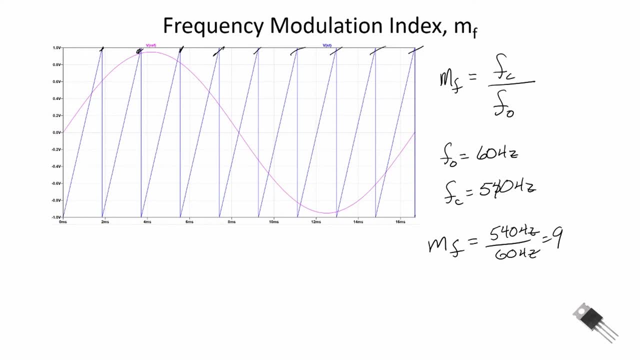 within one of our reference cycles. The other index I'd like to talk about is called the amplitude modulation index, And M sub A is equal to our reference maximum value divided by our carrier maximum value. And here we see: our carrier maximum value is one. 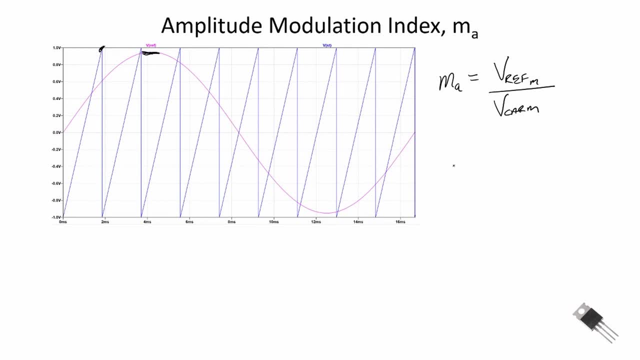 and our reference maximum value is about 0.95.. So for this example, M A is equal to 0.95.. I'm using volts, but it doesn't have to be 0.95.. If we're doing this in logic divided by one, 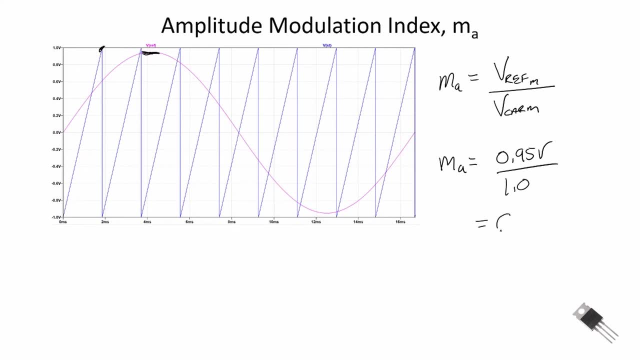 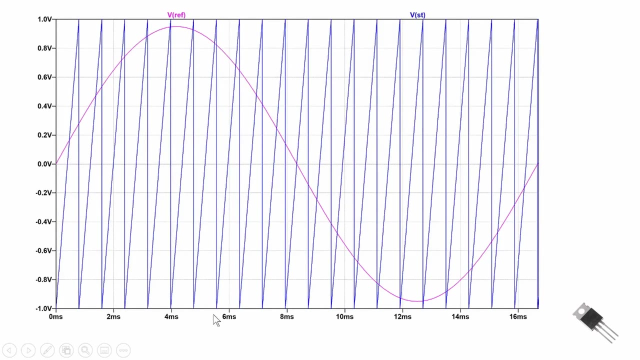 And so we have a amplitude modulation index for this example of about 0.95.. Now let's look at how we can control the frequency modulation index and the amplitude modulation index to get different resulting waveforms out of the load. So in this example I've increased the 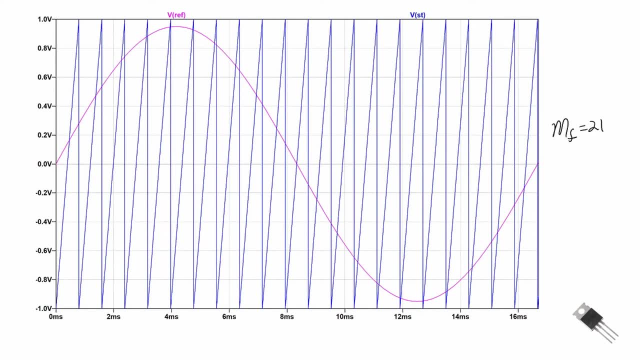 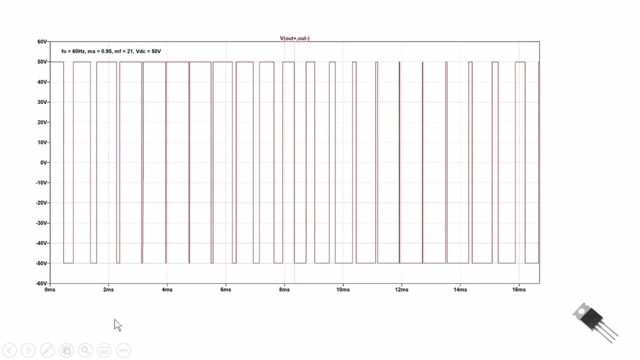 modulation frequency modulation index, and this is equal to 21, and one of the ways we can do it is just count the number of sawtooths when in within one cycle of our reference cycle and you'll see. if you count them up, it's 21. 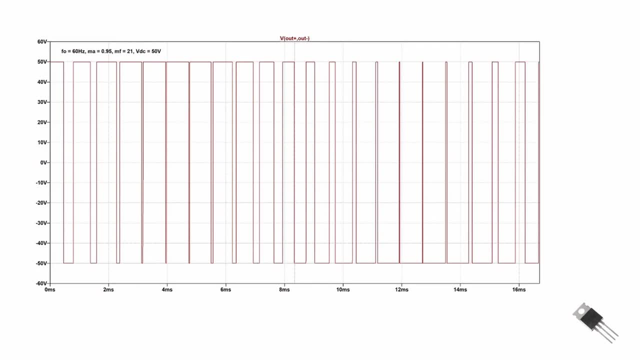 and here we can see a little bit how that changes our voltage across our load for our H bridge, and oftentimes our loads on our inverters are inductive in nature, so it's not so much the voltage that we want to think about, but it's the 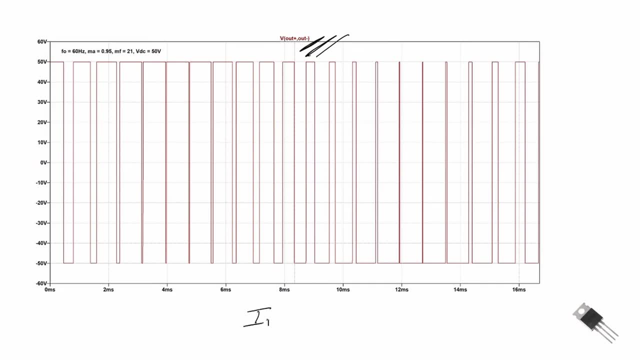 current through the load. so I Sabel is going to equal V Sabel and I'm going to do it in magnitudes because we're going to have harmonic content, and so we want to look at the current through our load as we change our our frequency modulation index. and here we have our frequency modulation index for: 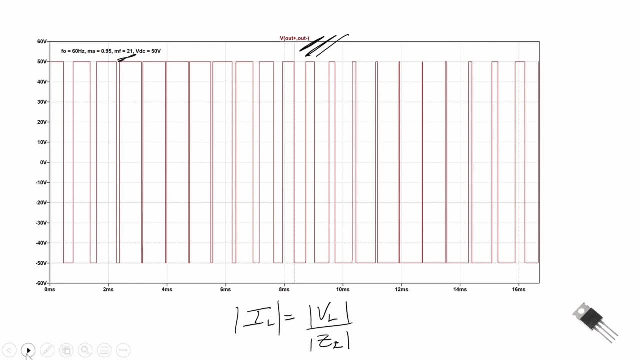 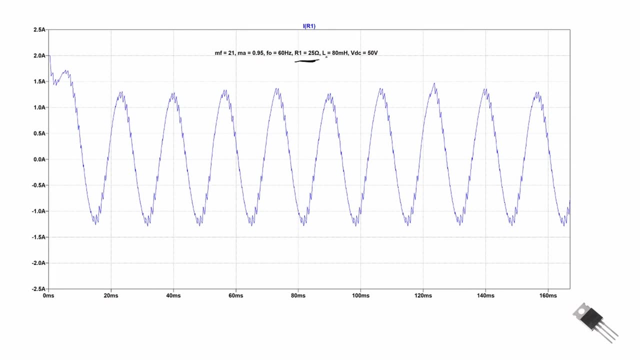 this example was 21, so here is the current through a load, and the load consists of a 25 ohm resistance in series with an 80 millihenry inductance. we have our modulation frequency index of 21. we have a 3.6 ohm resistance in series with an 80 millihenry inductance. we have our modulation frequency index of 21. we have our 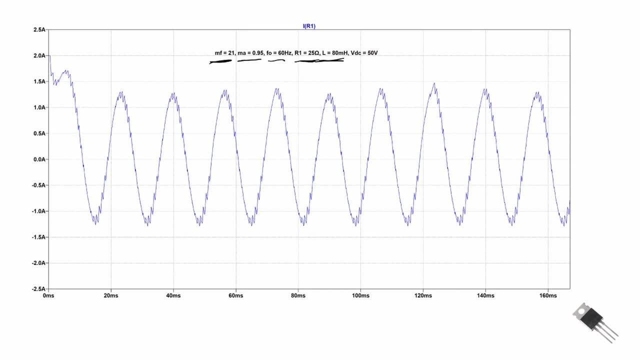 have an amplitude index of 0.95.. We're using a 60 hertz sinusoidal reference signal And we have our DC voltage of about 50 volts And you can see that we have our resulting current waveform through this load is somewhat sinusoidal. It's not perfect, but it's okay. And if I just did a quick, 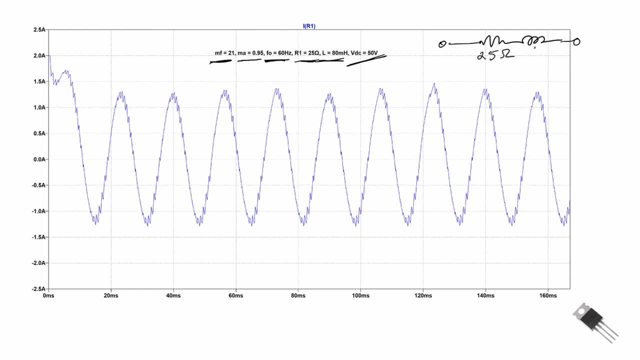 look at 25 ohms and ignored the inductance. 50 volts divided by 25 ohms is equal to 2 amps, And we're slightly less than 2 amps because the inductor is going to also have some inductance at 60 hertz. Matter of fact, it has, I believe, 37 ohms of reactance. 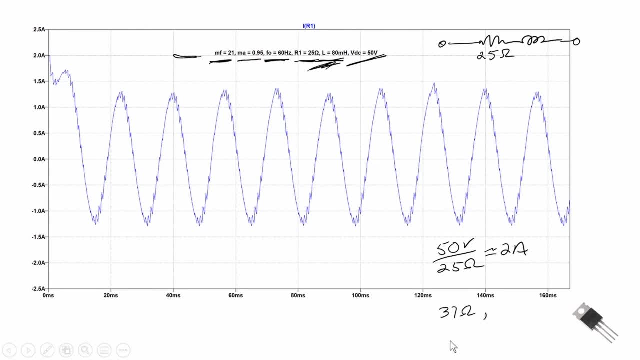 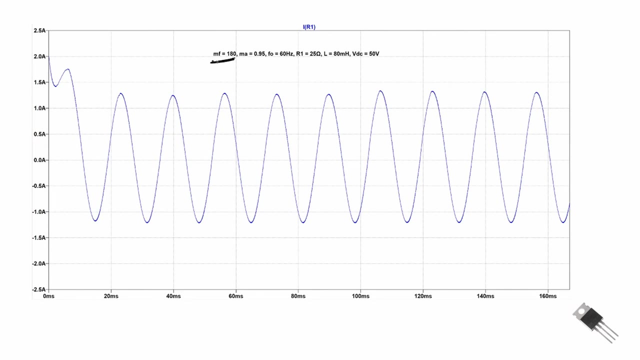 at 60 hertz. You can do the math on that one to find that out. Now let's change the index, modulation of frequency, And we're going to increase it, And here we've increased it up to 180.. And we've left all the other parameters for this problem the same. 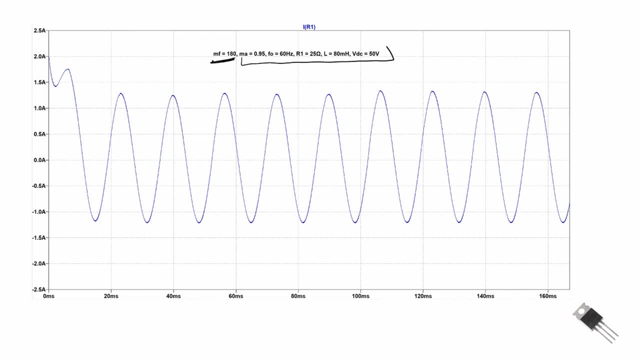 And right there you can see that the current through our series load across our H-bridge has really smoothed out. once we've used a higher index of frequency modulation- changing it from 21 to 180, has really smoothed out the waveform And we'll talk about that in a future video of why that is. 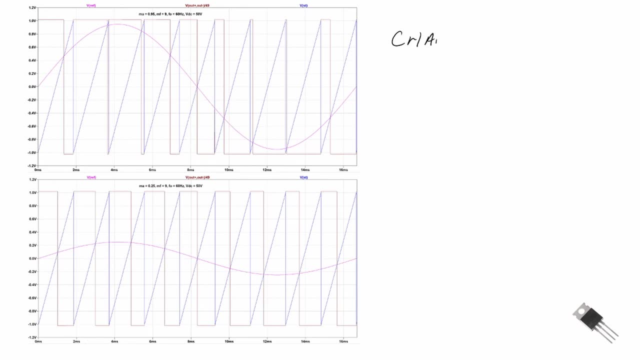 Now let's explore what happens when we change the frequency of the frequency modulation. So what happens when we change our amplitude modulation index? So here we have ma equal to 0.95. And here we have ma equal to 0.25.. And I've normalized our switching voltages across our H-bridge. 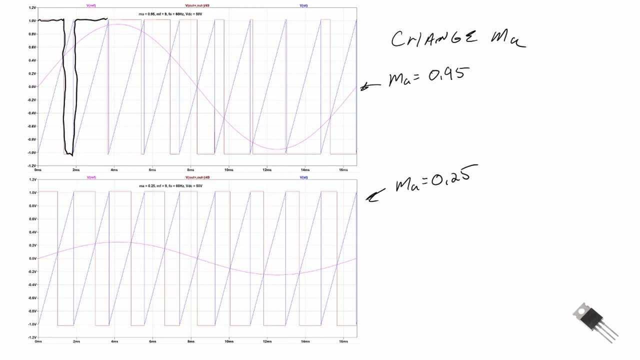 to fit on the same graph. So I've normalized them close to one volt so that we have a peak And you can see as we decrease our modulation index. the average duty cycle gets closer to one half and stays very close to one half. 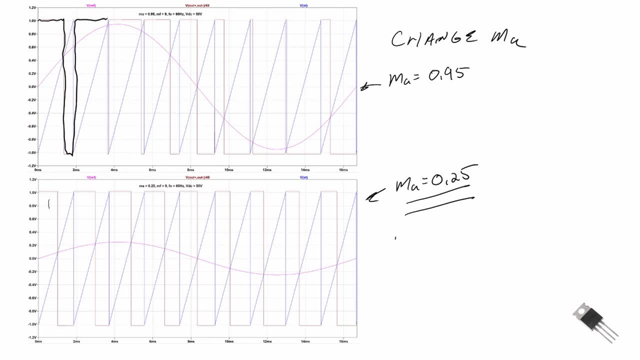 As a matter of fact, if we let ma equal 0,, the duty cycle on our switching voltage across our waveform would exactly equal one half, because our reference signal, which is our H-bridge, is exactly equal to one half. So we have the same frequency as our H-bridge. 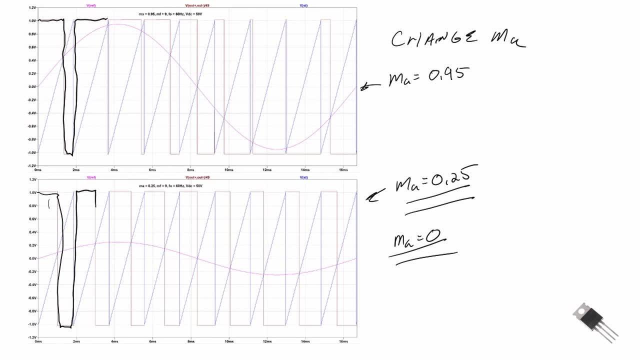 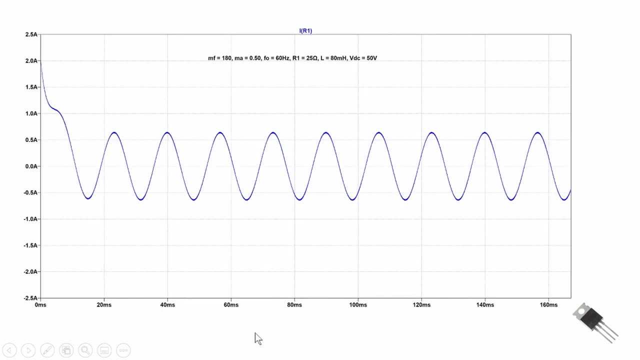 signal would be above our carrier- our sawtooth carrier- half the time and below our sawtooth carrier half the time. Let's investigate that as we apply it to our load. and here we have. we'll continue with our index of modulation for frequency at 180. we have our 60 Hertz load, we still have our 25 ohm and 80. 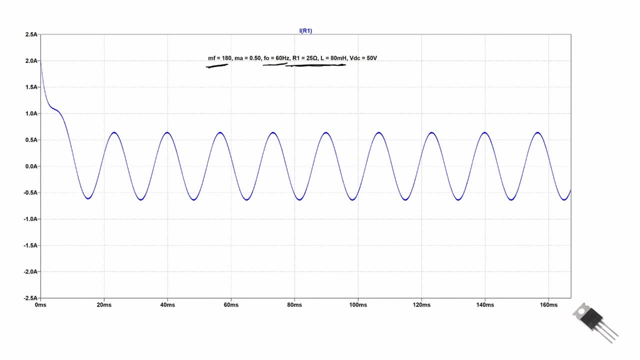 millihenry series and load across our H bridge and we're switching back and forth at plus 50 volts and minus 50 volts across that load and here is the resulting current and we can see that that is about. oh, that's got about about. 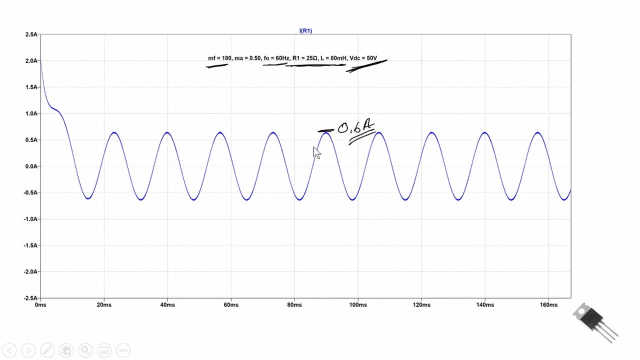 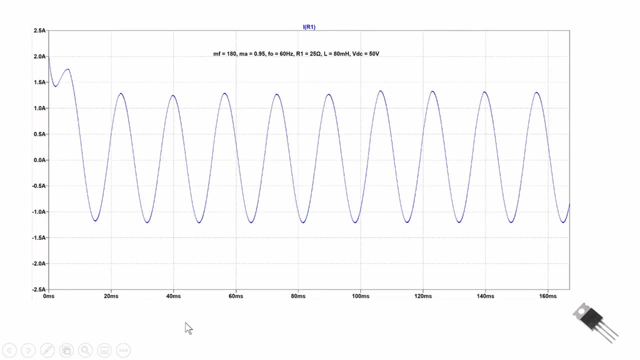 a point six amp peak value. and now let's change our index of modulation for amplitude, our M sub a. Here we've increased it to 0.95 and we see we went up from 0.6 amps to about 1.2 amps or 1.25 amps by by changing that so we can control the amplitude of the. 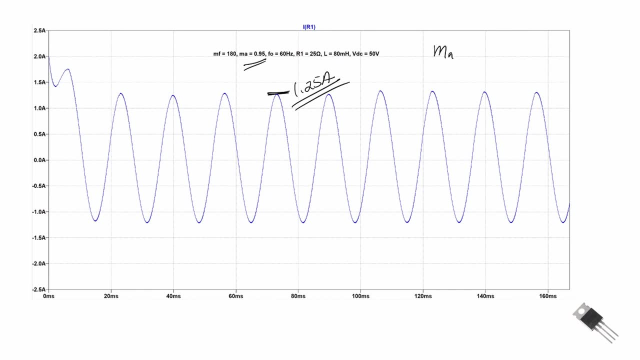 current through our load by controlling M sub a. and the way we control M sub a is by controlling the amplitude on our reference signal. we can control this frequency by controlling the amplitude. by controlling the frequency of our reference signal, We control the amplitude by controlling the amplitude on reference signal. that's 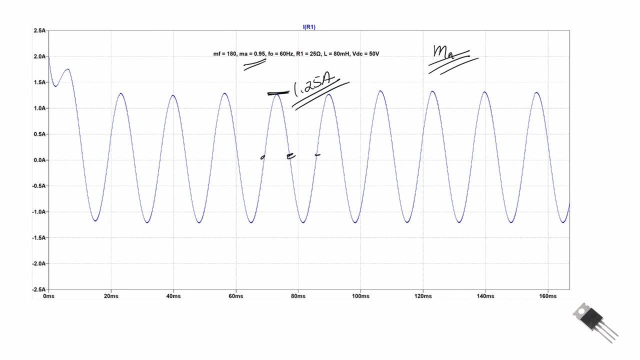 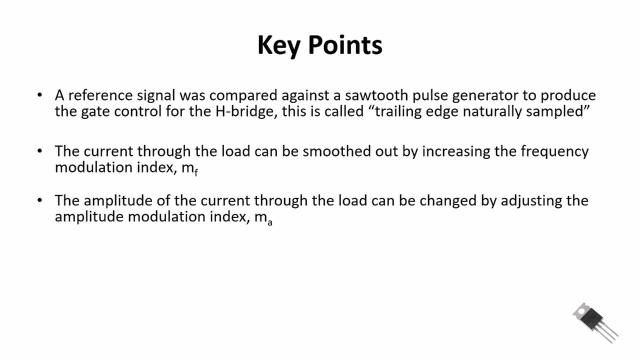 important because if I can control frequency and the amplitude of current through motor, I can control speed and torque that that motor delivers. So let's recap the key points. and for this H bridge it was called a trailing edge, naturally sampled, and there are other types of PWM configurations. 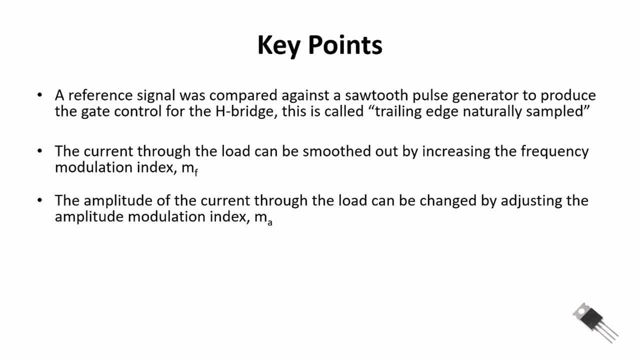 But this is one of the easier ones to to help with introduction to PWM inverters And we compared a reference signal against a sawtooth pulse generator and that's what we use to control the H bridge. and we looked at two parameters. the first one was the frequency. 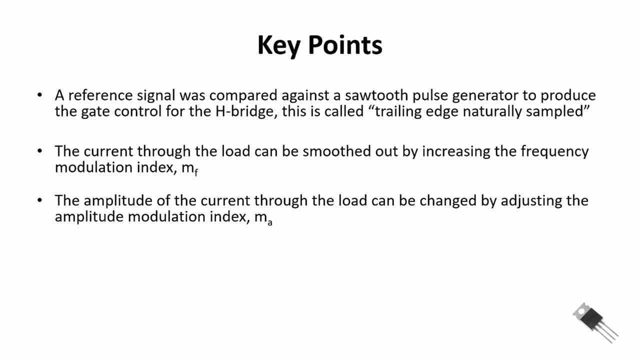 modulation index M sub f and that smoothed out the current through our load by increasing it. And then we also looked at the amplitude modulation. So we looked at the frequency modulation index M sub f and that smoothed out the current through our load by increasing it. And then we also looked at the amplitude modulation.